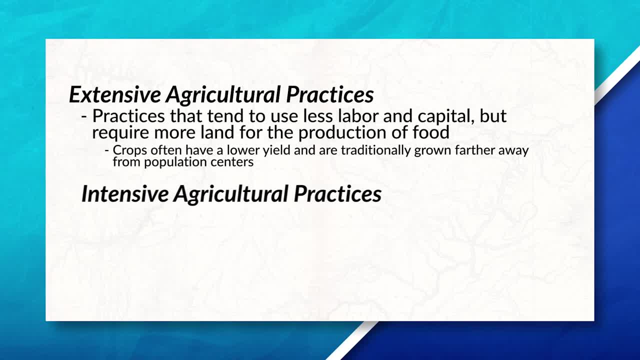 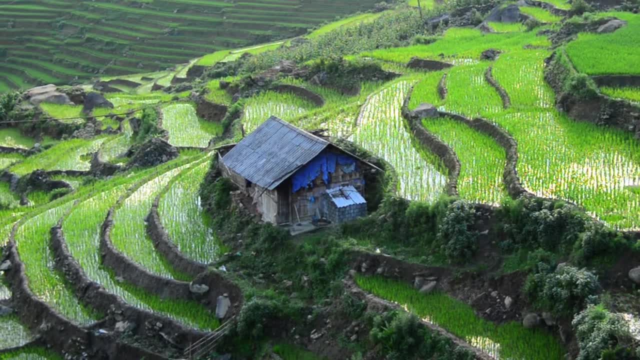 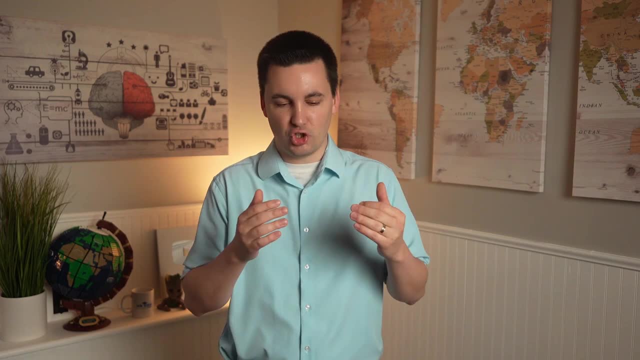 agriculture would be pastoral nomads. Intensive subsistence agricultural practices, on the other hand, tend to use less land, more human labor and may require more capital, Such as intensive subsistence with wet rice farming and terracotta. If we look at agricultural practices that generate revenue, we can see extensive commercial. 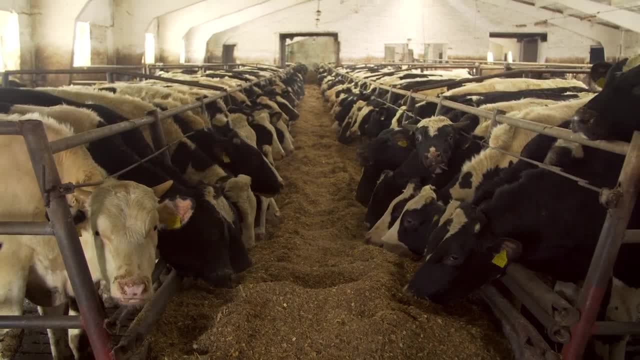 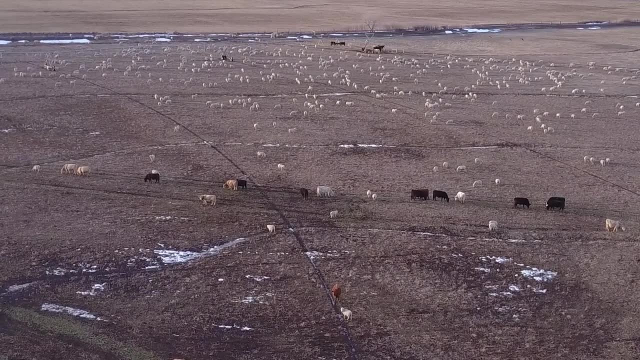 agricultural practices which traditionally use less capital, machines and human labor, but often do require significant amounts of land, Such as cattle ranching, which uses few machines and lots of land and has a goal of making a profit off the cattle that are raised. Lastly, 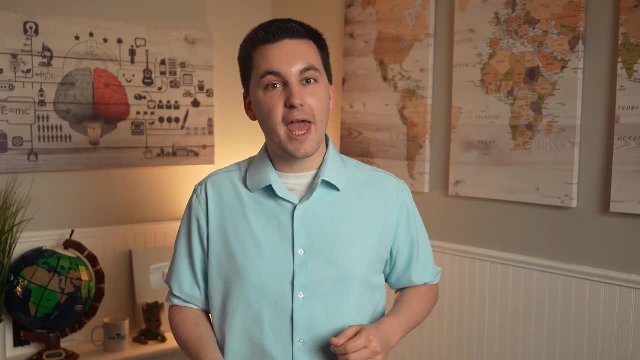 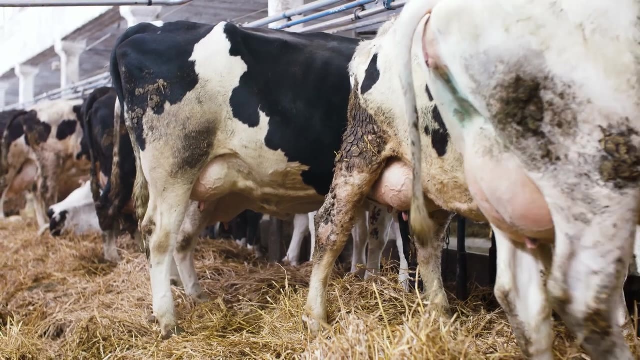 there is intensive commercial agricultural practices which use less land but more capital, machines and or human labor, For example, dairy farming, which requires a significant amount of work, of having the cows being milked at least twice a day, and lots of investment to purchase the machines needed for large scale production. 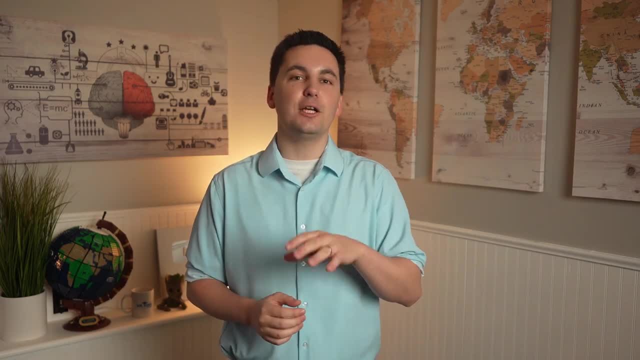 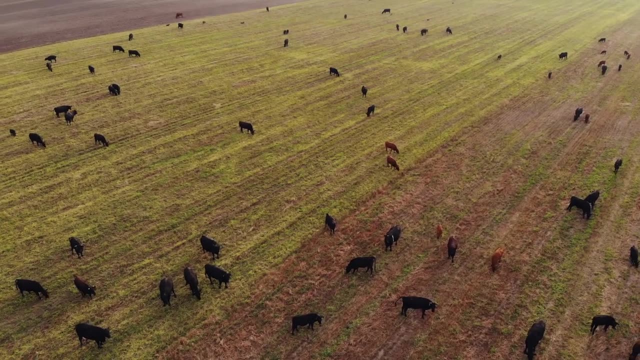 Often times, we see agriculture that is intensive located near a market or city, while agriculture that is extensive and needs more land will be located farther away from a city or market. This is partially due to the bid rent theory, which is an important theory that will 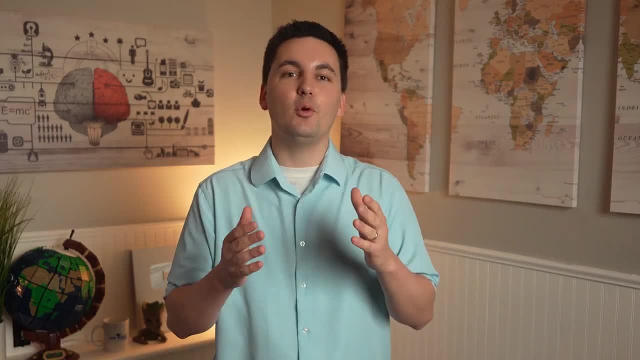 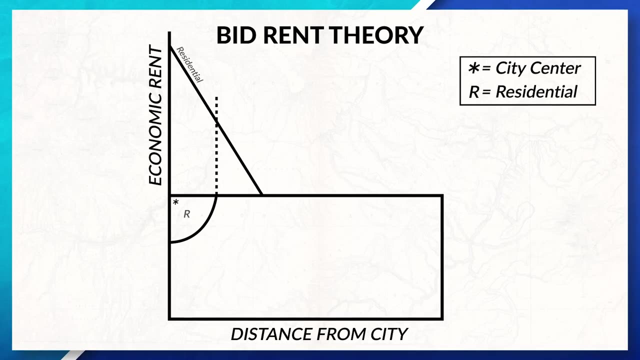 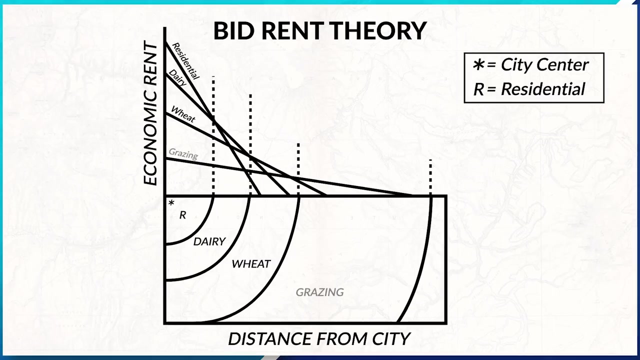 come up later in this unit when we talk about Von Thunen, And again when we go into our unit 6 and look at the price of land in relation to the city or urban area. As we move further away from the city, we see the price of land go down. However, as we get closer to the city, the price of land 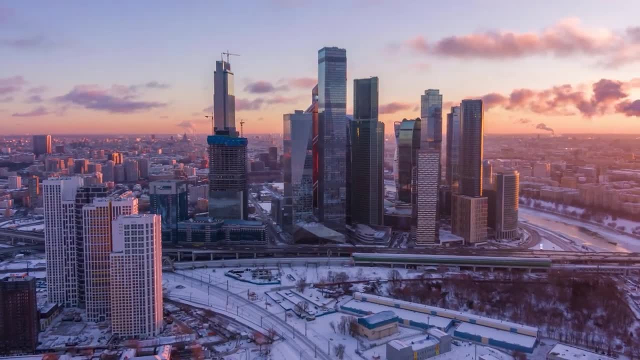 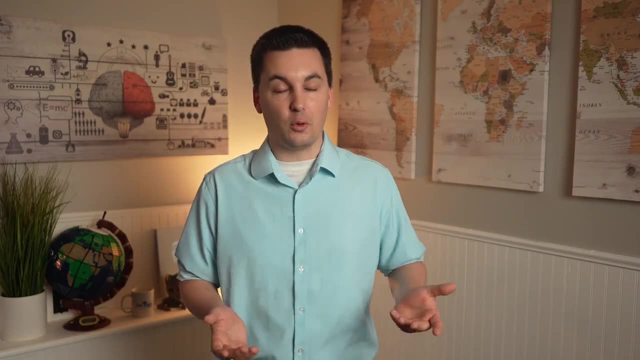 goes up. This is all because of scarcity. Cities have less land available due to the higher population density, so the cost of land is more. As we move farther away from the city, the demand for land goes down, which means more land is available, thus decreasing the price of land. So 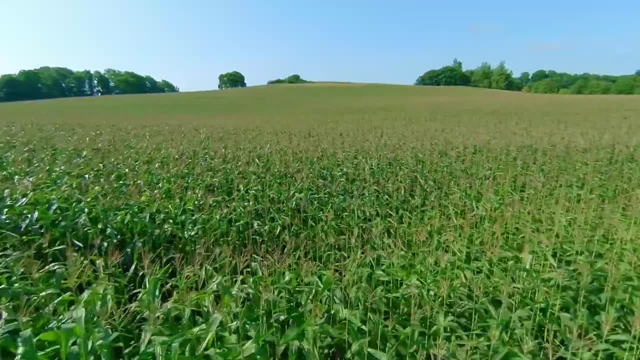 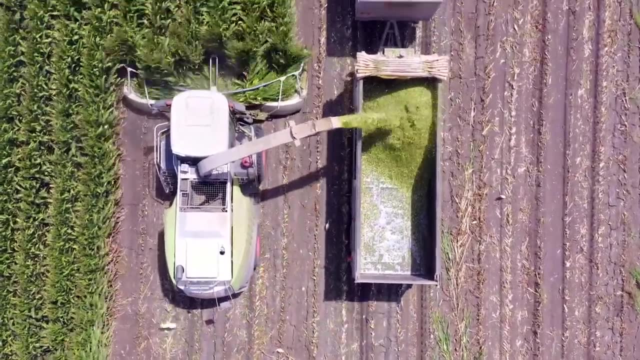 agriculture that needs more land is often located farther away from an urban area. To take advantage of this, we can see that the cost of land is higher and the cost of land is lower. This is especially true if transporting the final product is relatively inexpensive. 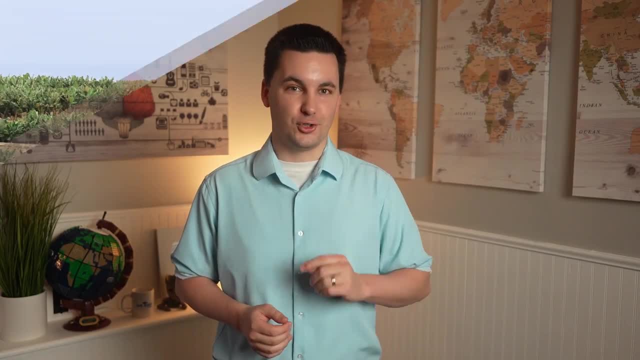 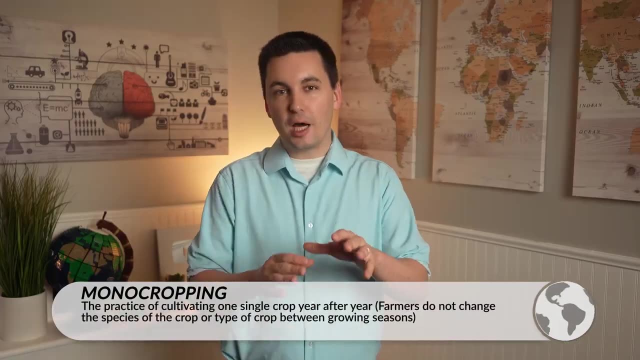 Today, we can also see the impact of monocropping and monoculture. Monocropping is when farmers grow the same crop each year. They continue to plant the same species of crop year after year after year. Now, monocropping does risk soil depletion due to the lack of crop rotation. However,